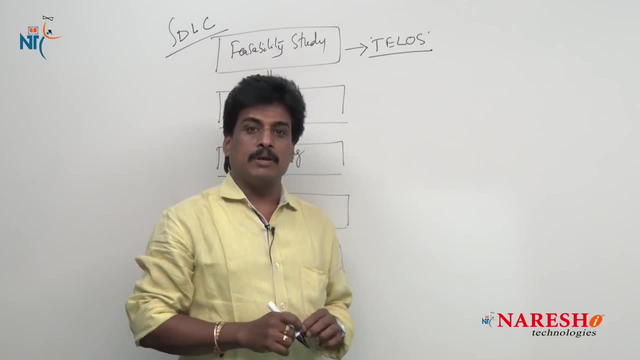 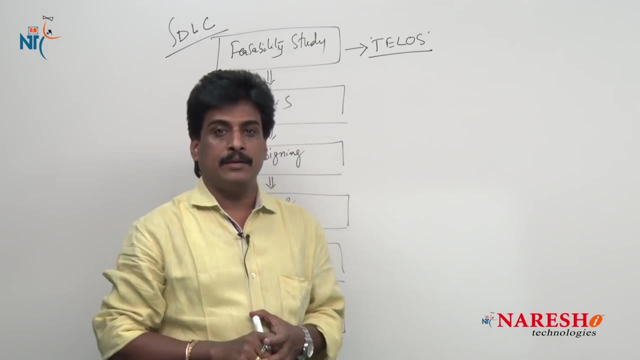 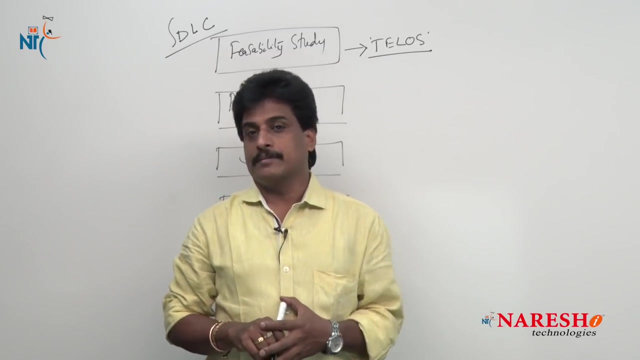 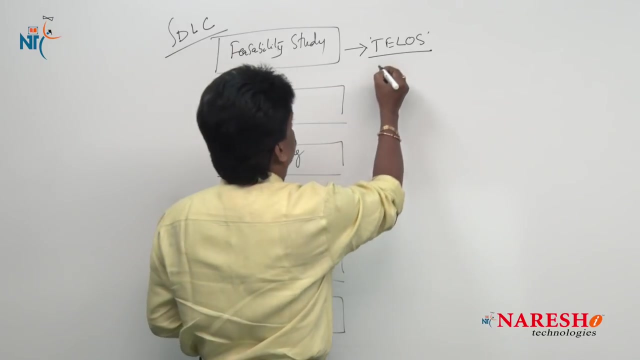 T stands for technical feasibility, E stands for economic feasibility, L stands for legal feasibility, O stands for operational feasibility, S stands for schedule feasibility. So this is TELOS. We can able to view in detail, one by one, Technical feasibility. What exactly, the meaning of technical feasibility? 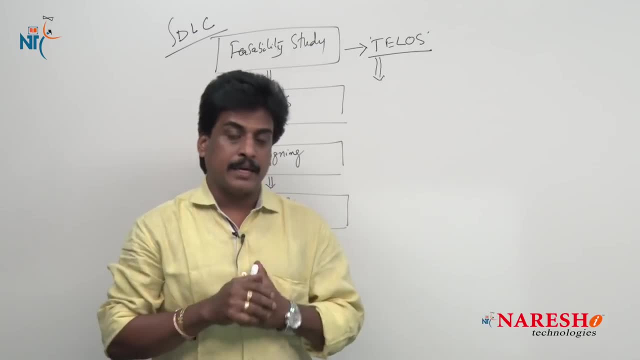 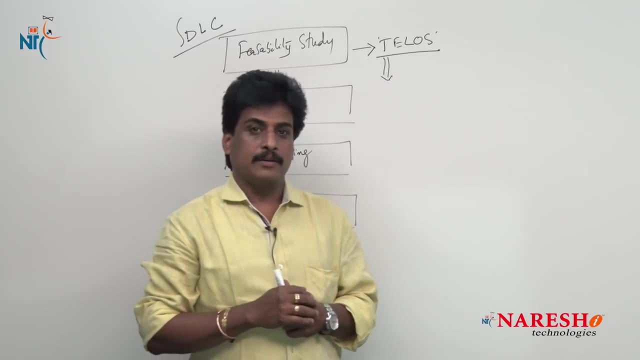 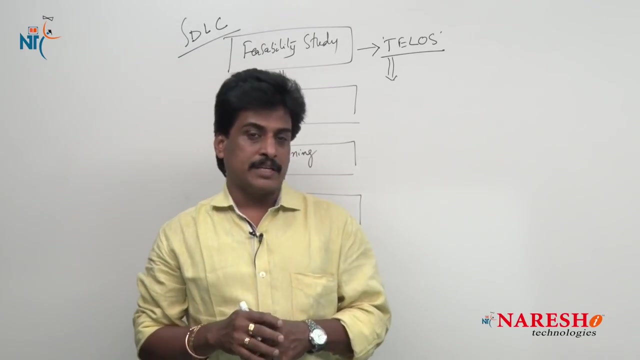 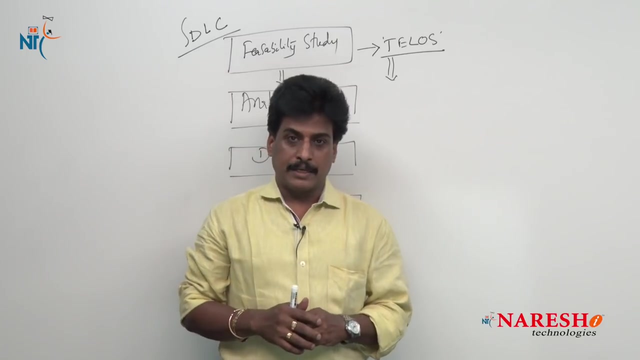 As per the client requirement, the company thinking For software and hardware requirements, as well as staff members. all these are perfectly existed or not. Economic feasibility: Whatever the budget is there within the budget, can we complete the project or not? And next one is legal feasibility. 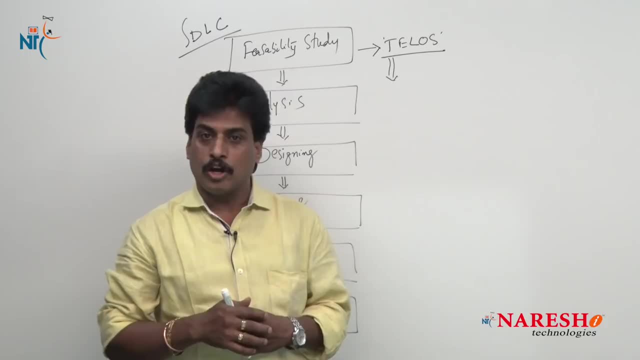 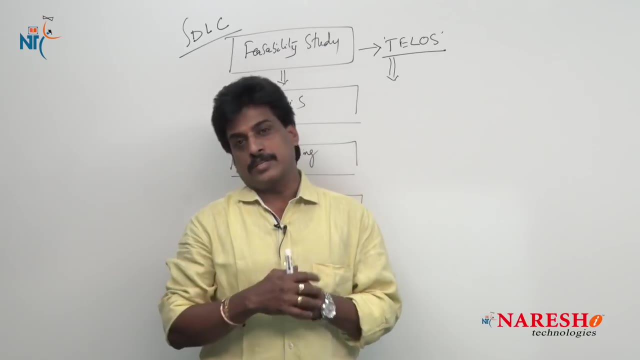 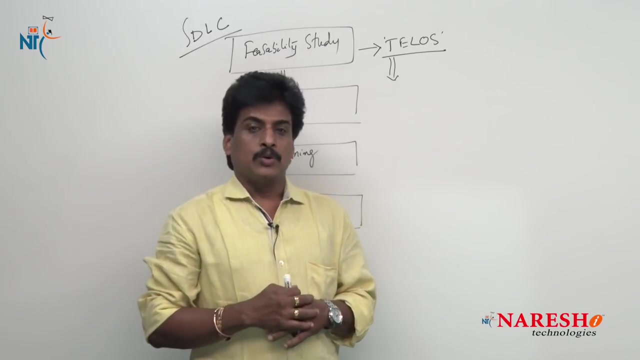 As per the rules of cyber law. can we handle that or not? Operational feasibility: Whatever the client or client users expecting, Those operations, can we develop? can we explain that and these are and finally schedule within the time whatever client expecting, can we able to deliver or not? 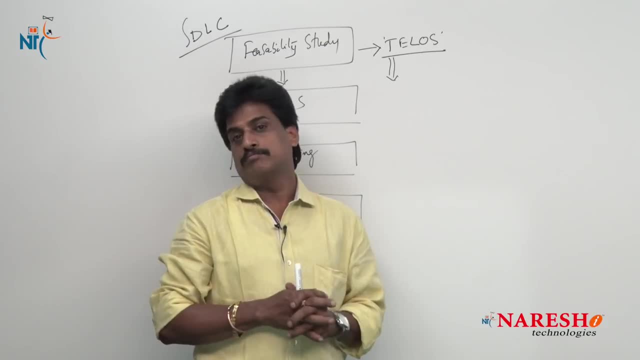 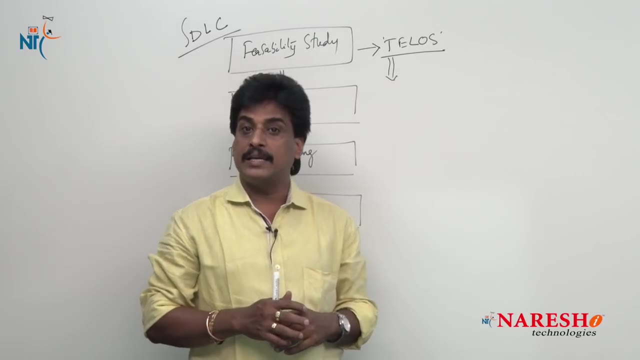 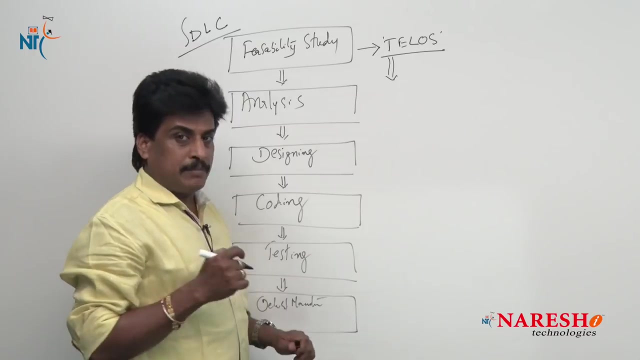 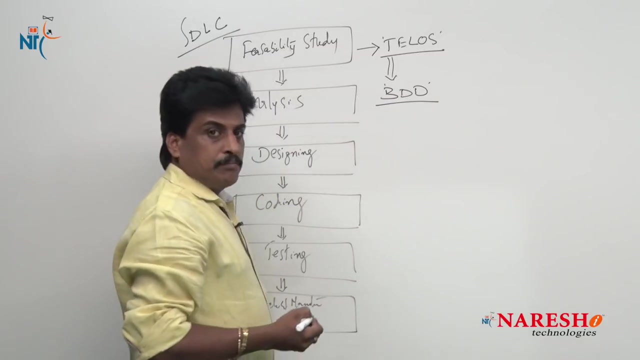 So these are the main things actually we need to perform. So TELOS is very powerful formula which is existed in the feasibility study environment area. So once TELOS successfully completed, Once business requirements Successfully gathered, gathered requirements are writing in a separate document is called business design document BDD. 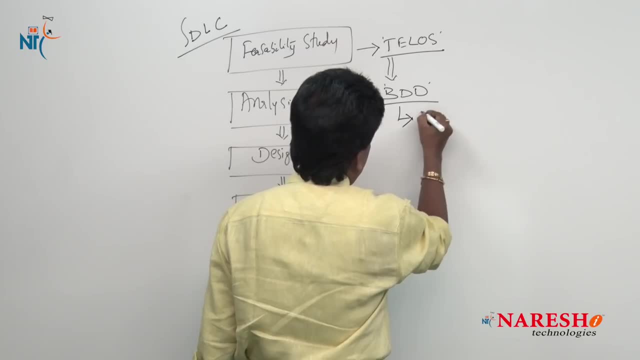 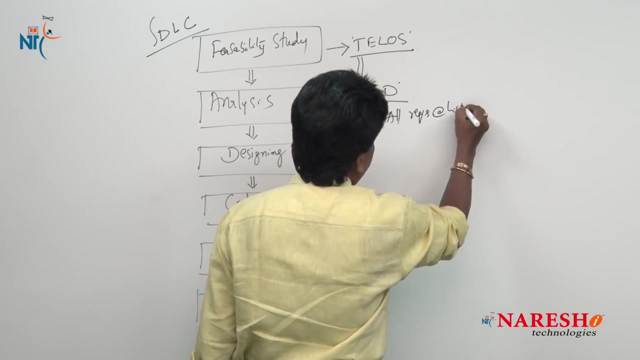 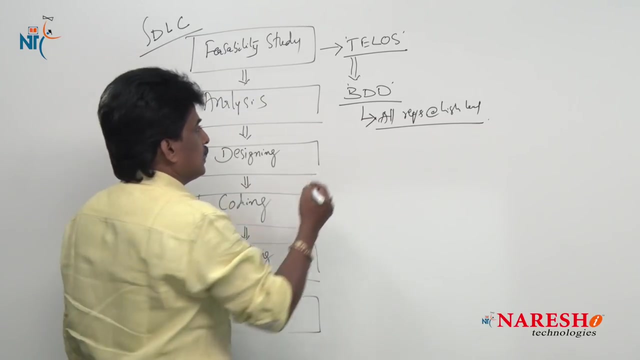 So in this business design document, all the requirements available, all the recs existed at the high level. So these requirements as a technical member we are unable to understand At that time. this is one input document to next phase. So what are the input here? 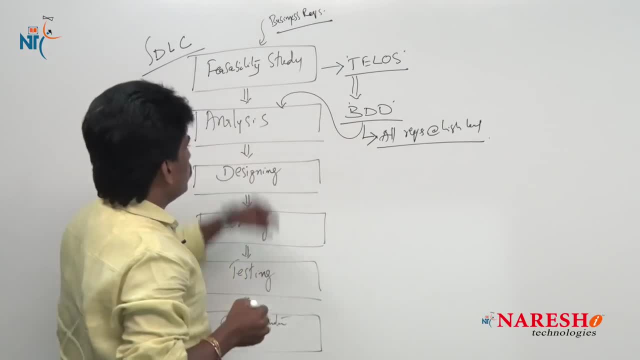 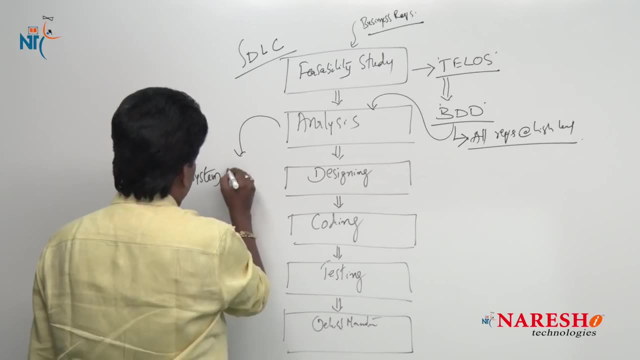 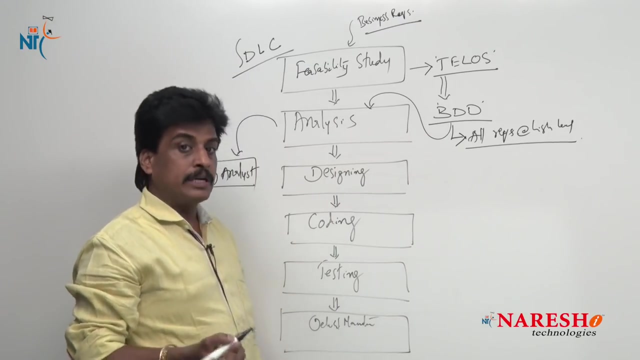 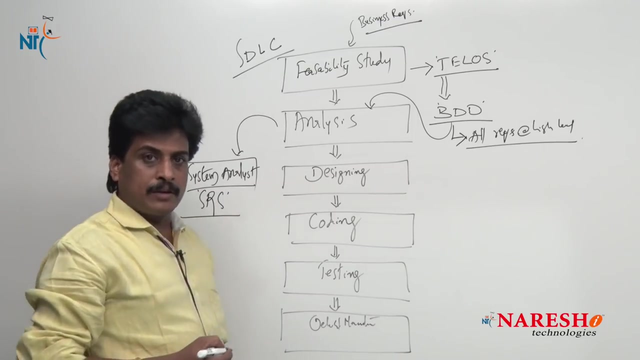 Business recs. So that is input and BDD is input to this one. So in this analysis phase, system analyst, involving System analyst, all business requirements converting into technical requirements in the name of SRS document, Software requirement specifications or system requirement specifications. 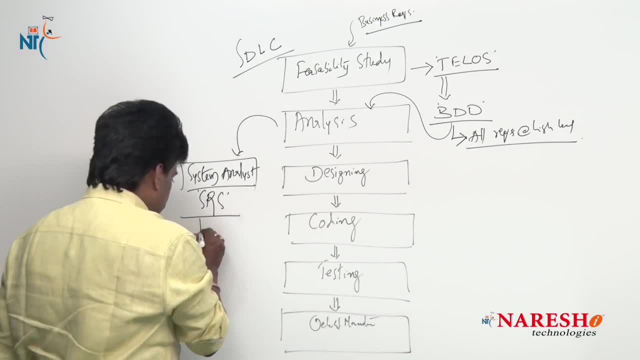 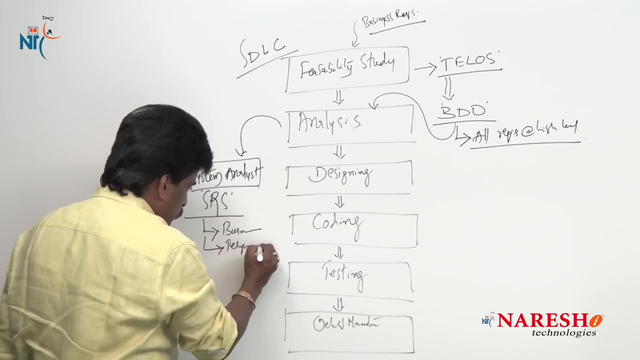 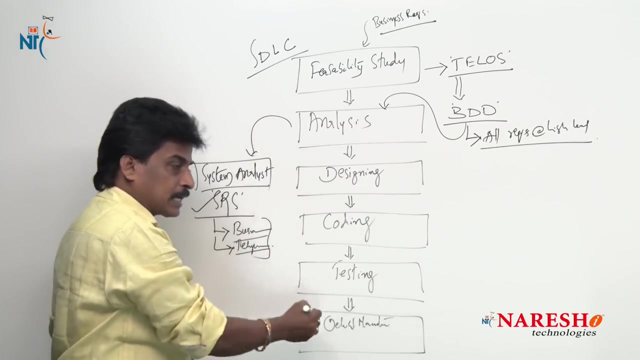 So these are the. this is the document where exactly business requirements existed, as well as a technical requirements also existed, So both the requirements available. It is a crucial document in entire the project life cycle, So it contains a business requirements, So both the requirements available. 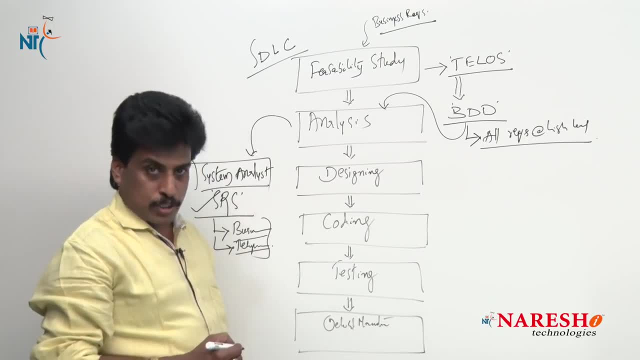 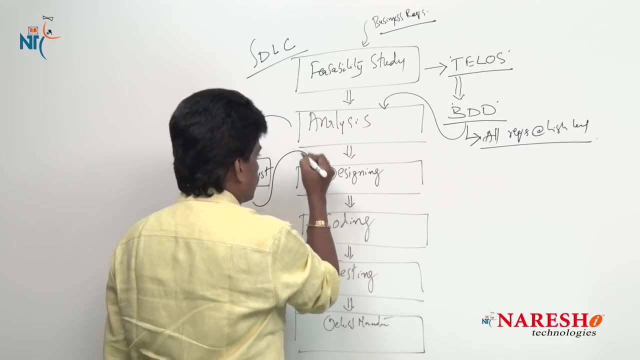 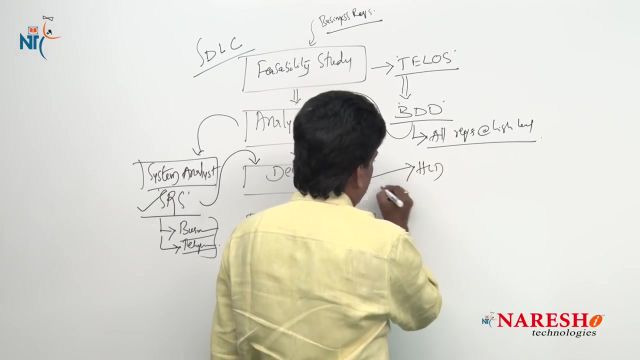 It is a crucial document in entire the project life cycle: Business requirements that related technical requirement solution. So done by this system analyst team. So this is the document input to the designing phase. Again, the designing is done in two levels: High level designing as well as a low level designing. 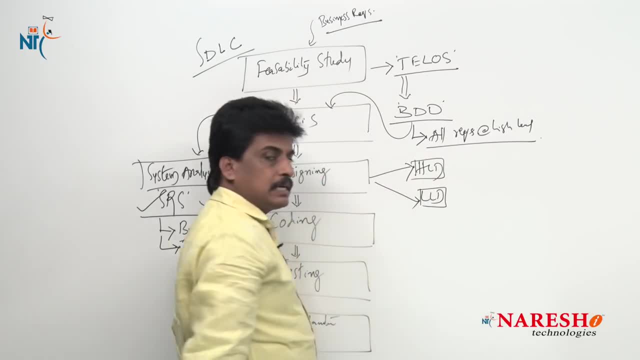 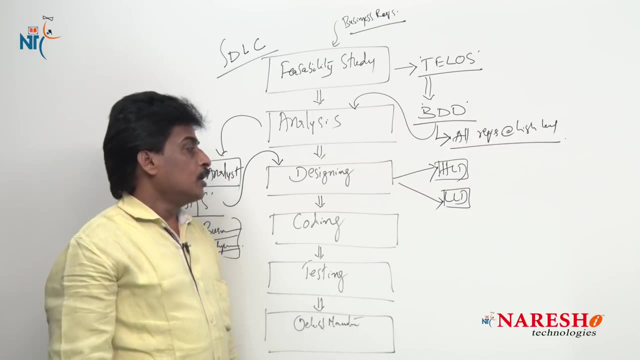 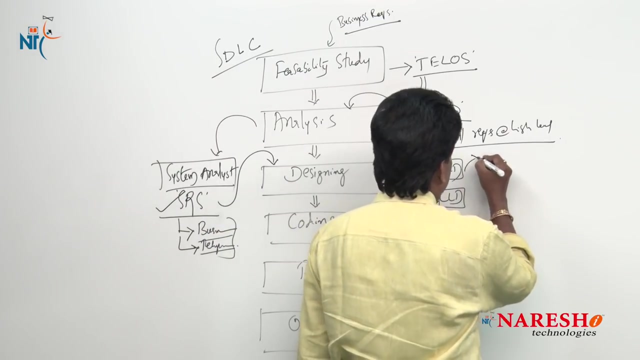 So what exactly low level designing? What exactly high level designing, Right High level designing environment. What are the things we are expecting Low level designing environment? What are the things we are expecting, For example, high level designing means what Main modules? 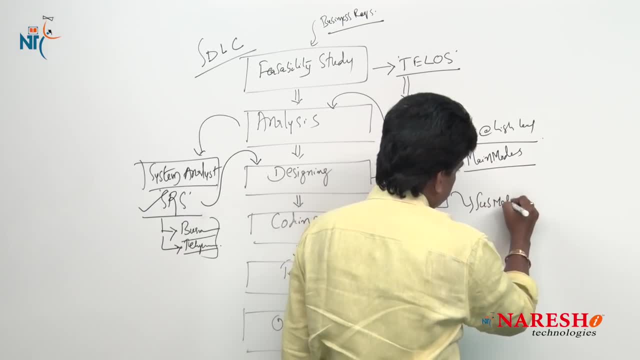 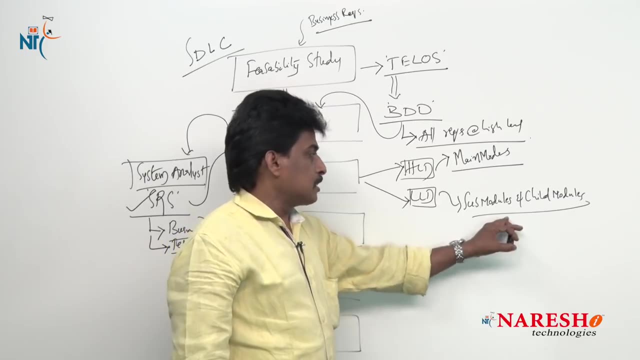 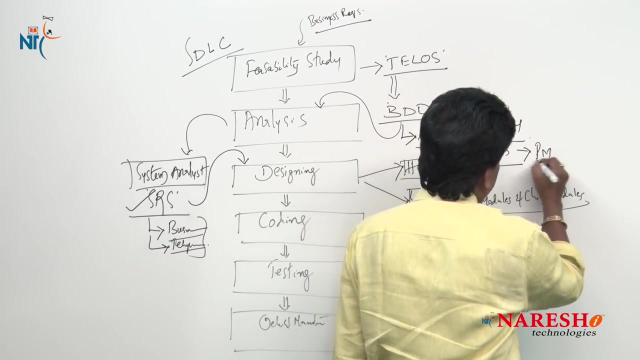 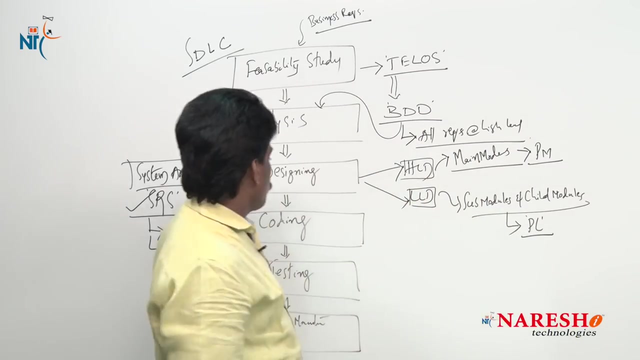 Low level designing means submodules and child modules. So main modules means high level designing. submodules and child modules are nothing but low level designing. It is always done by the project manager CADR people, It is always done by the project leader people. so it is what exactly designing meaning? so in this, in this. 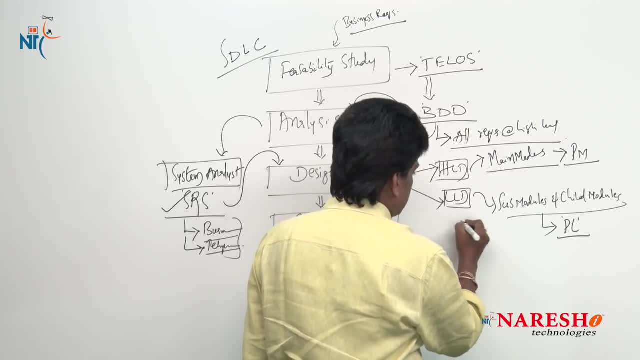 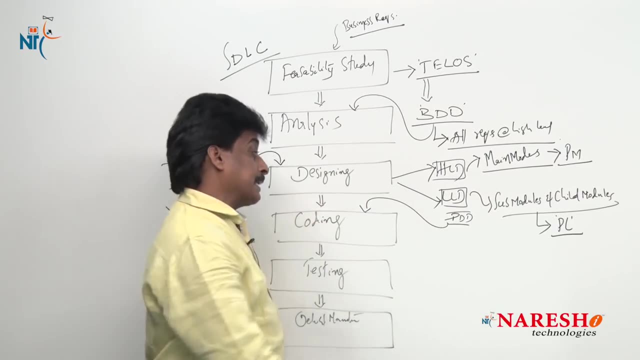 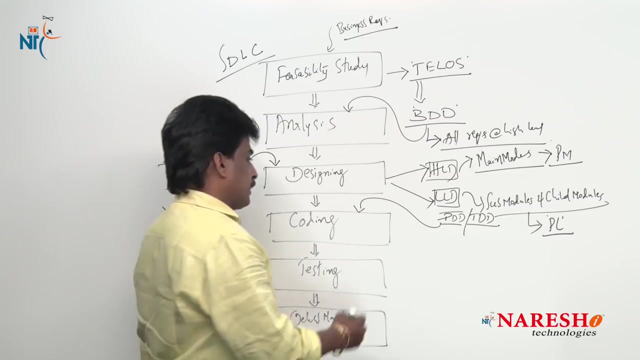 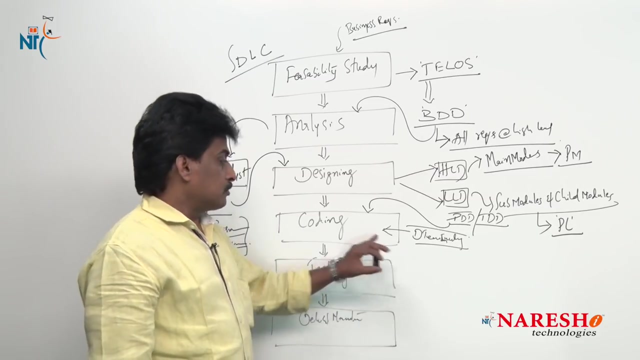 phase and there is a document existed. the document is nothing but project design doc, so it is input to the next phase or technical design document- different, different alias names available. it is input to the coding phase in this phase: total development team. involving development team. involving this development team developing total source. 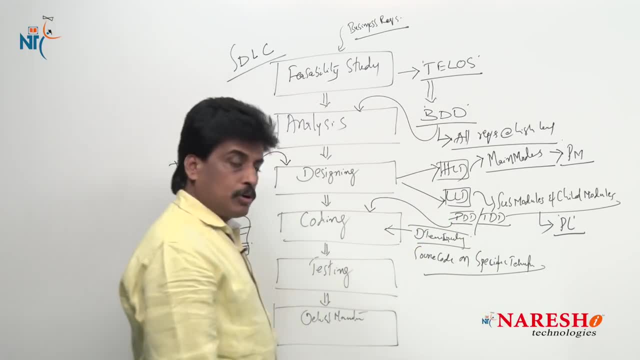 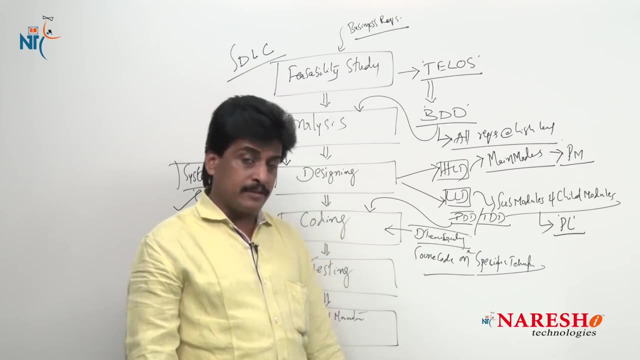 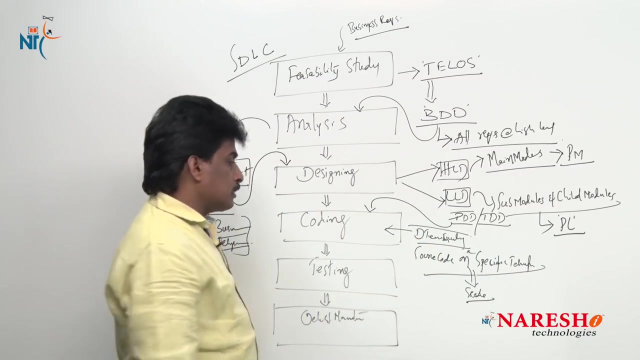 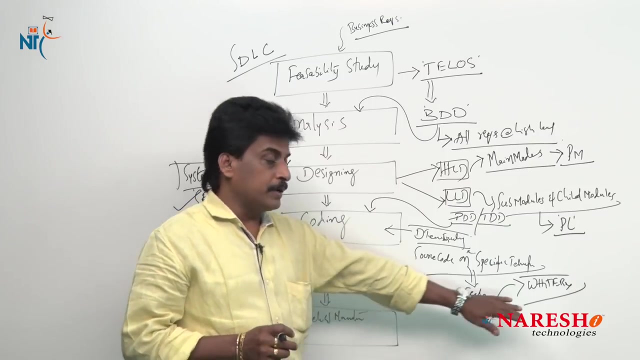 code, total source code on a specific technology like java, php, dotnet, python, like that. there is specific environment area. they are implementing source code. once they are implementing source code on the specific technology they are performing here, white box testing- okay, white box testing always done by the software developer or software engineer. it never performed. 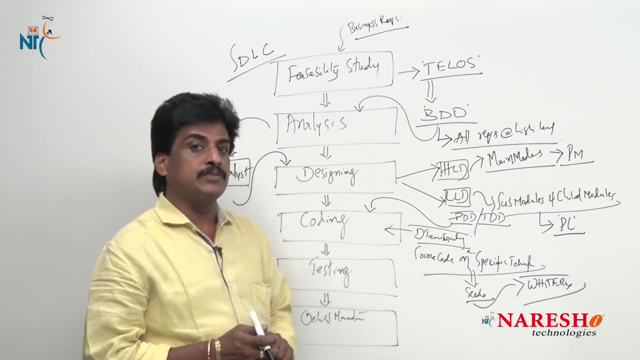 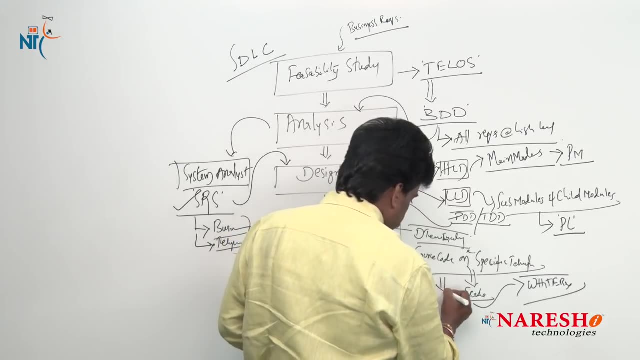 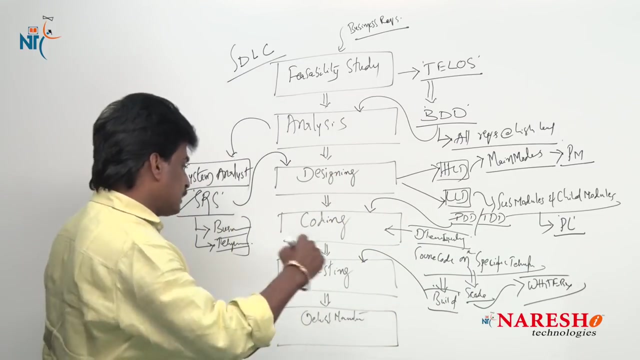 by any test engineer. one successful completion of the white box testing. it is coming to black box testing. so from this phase released one is nothing but build. the build is input to the testing team. then on that build there is a life cycle will be applied here the testing. 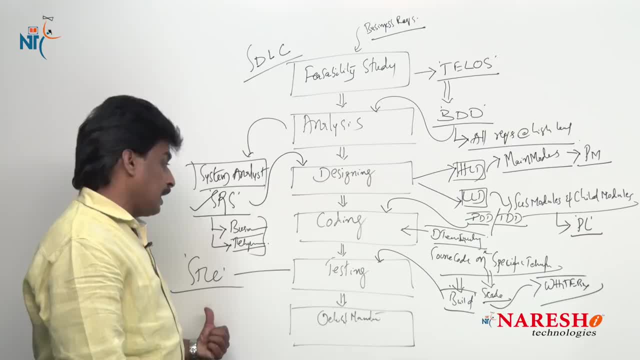 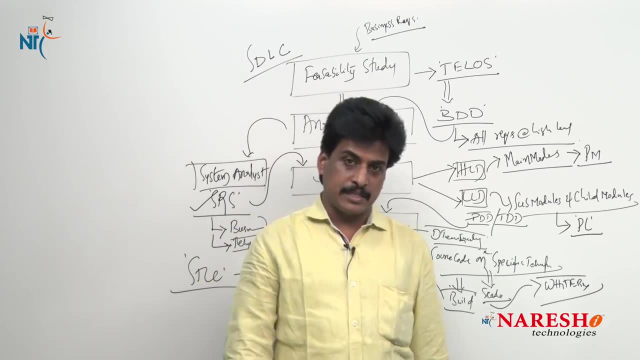 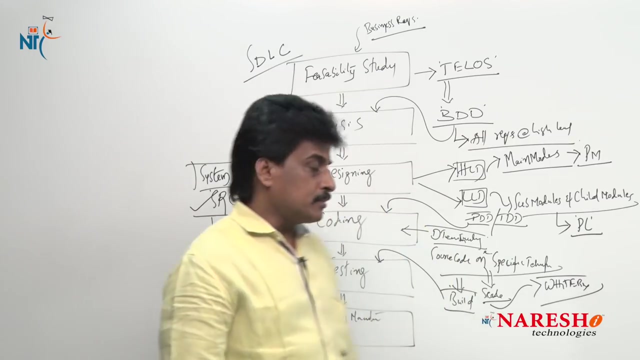 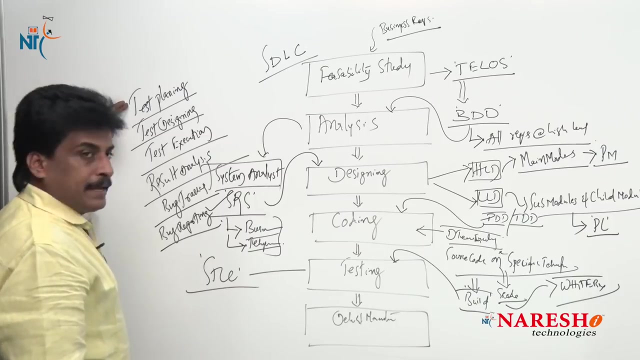 is called stlc software testing life cycle. again, it has six spaces: test designing, test planning, test designing test execution result analysis, bug tracking, bug reporting. so what are these six faces? we can try to observe one by one. so stlc contains test planning, test designing, test execution result analysis, bug tracking. 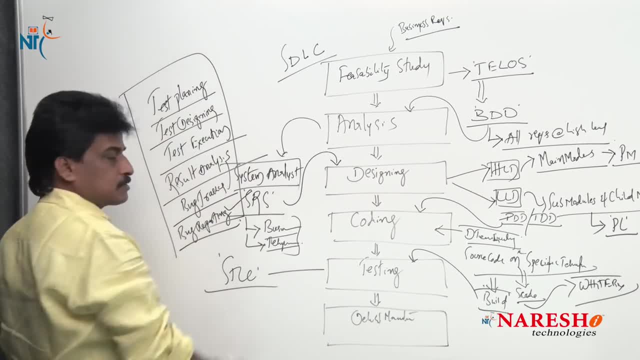 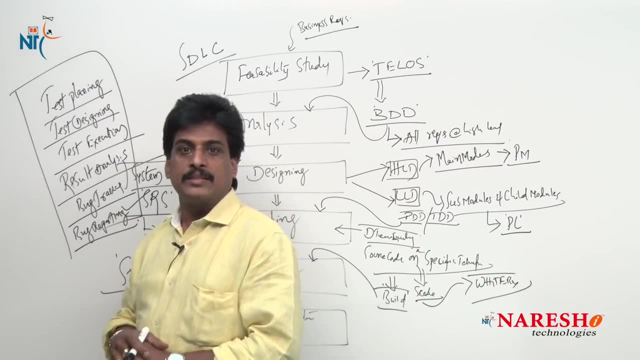 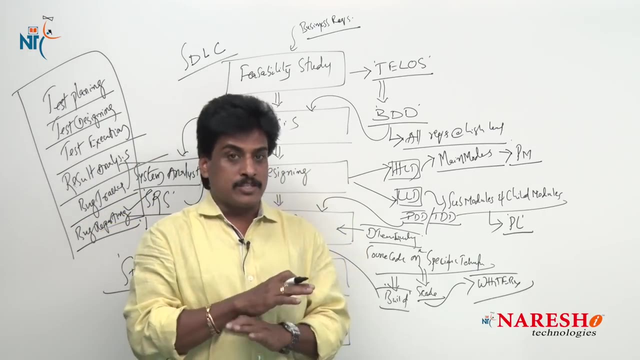 bug reporting. so these are the six phases exist, every phase important, every phase perfect. so these are the things. what exactly existed in the stlc manner. so sd stlc is one of the components under sdlc, so it is not a separate. so once you are trying to understand, system development life cycle. 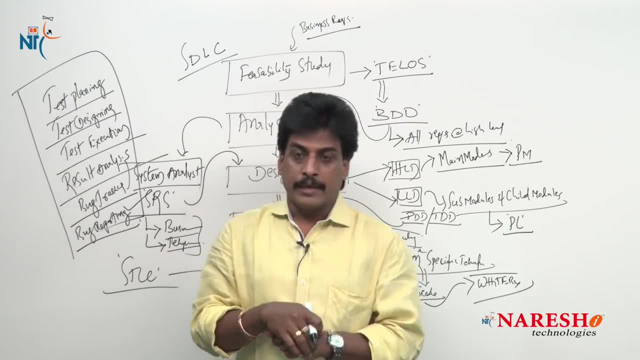 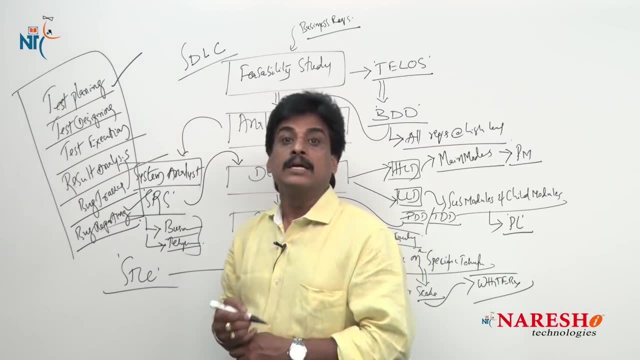 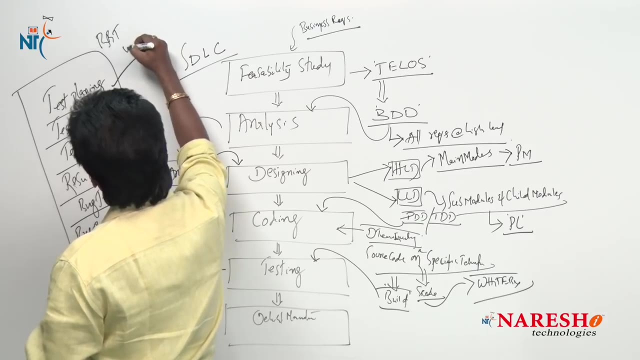 it contains even stlc components. also, again, test planning is a bigger one, so one by one i need to discuss means separately. i'll discuss in the next video session about the stlc and once testing successfully completed, it is completely black box testing life cycle. black box testing life cycle. 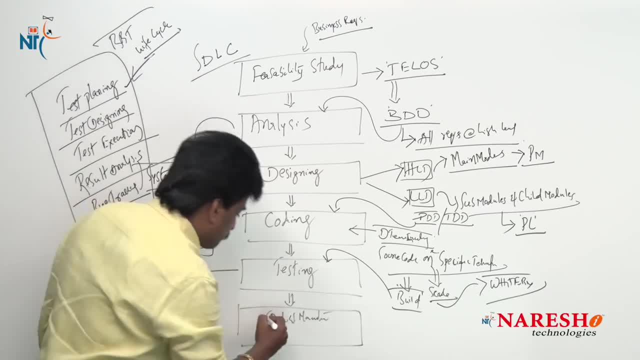 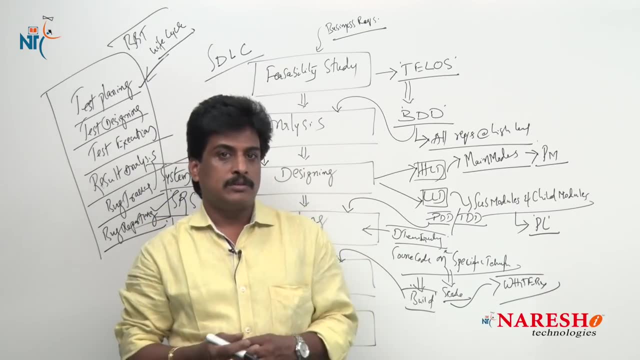 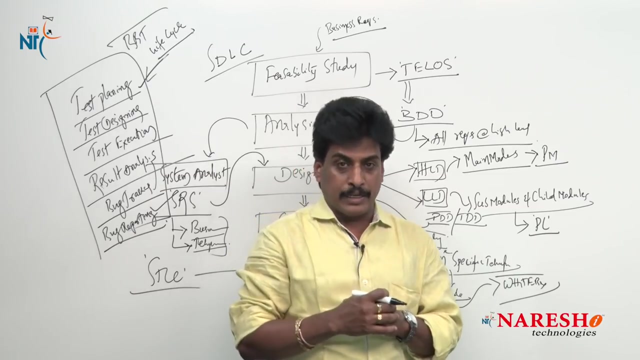 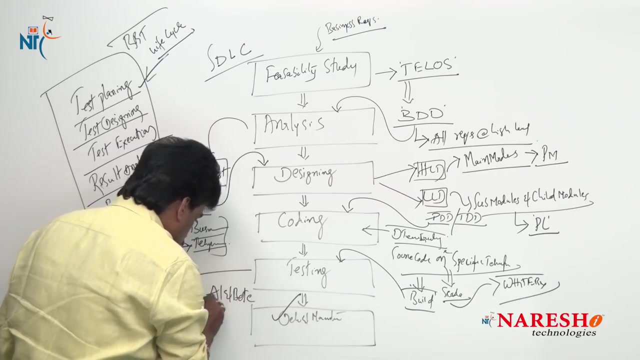 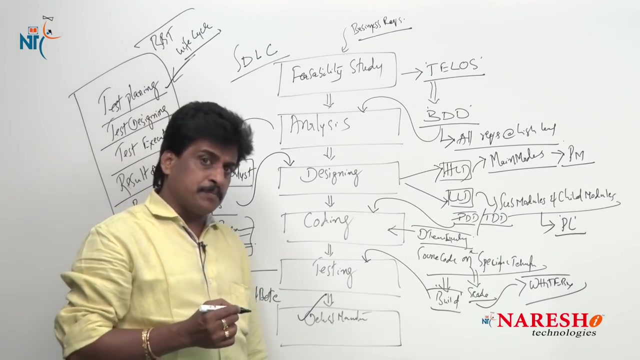 once testing successfully completed, then the next part is nothing but delivery. successfully tested project is we are ready to giving to the concerned client or concerned customer. that is called delivery. before we are going to delivery we must know what exactly that. that is alpha testing and beta testing. these two we are calling as user acceptance testings. what are user acceptance testings? what? 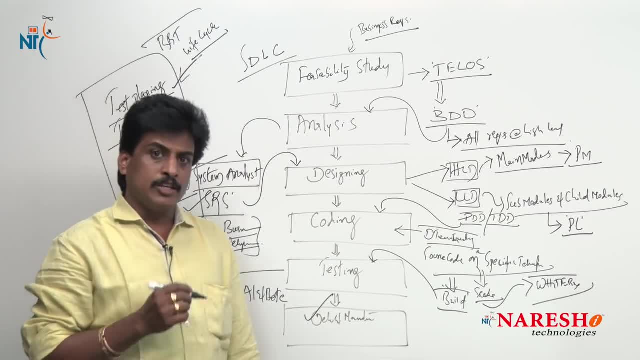 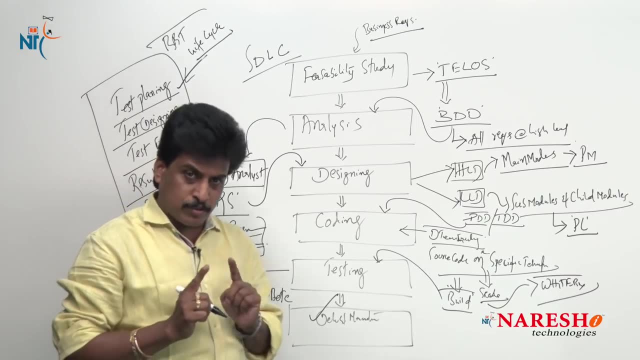 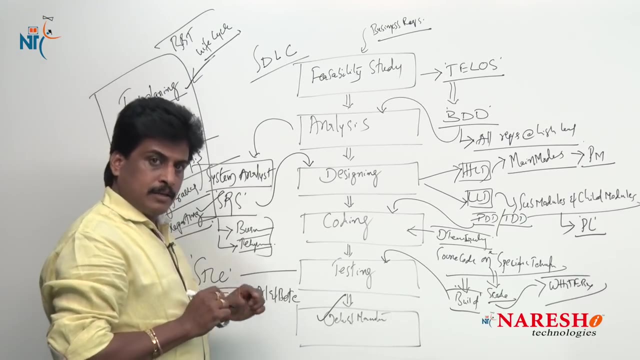 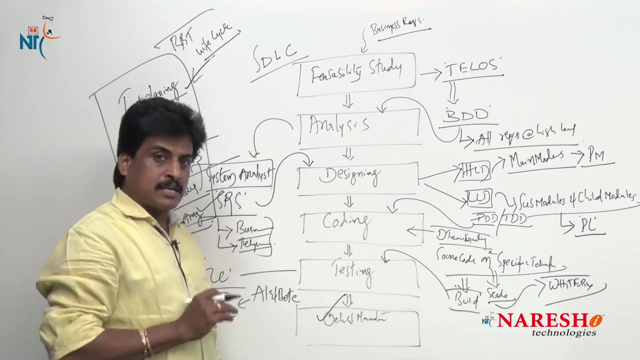 exactly happened here. so we'll try to understand once again user acceptance testing meaning. so user acceptance testing is nothing but one point. we need to remember here what that first we need to know what is alpha. for example, project completed, defect-free testing, also completed. now one successful testing completion- a client member is coming to company level. they are. 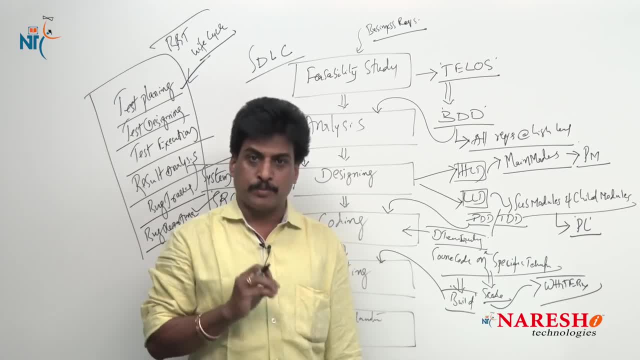 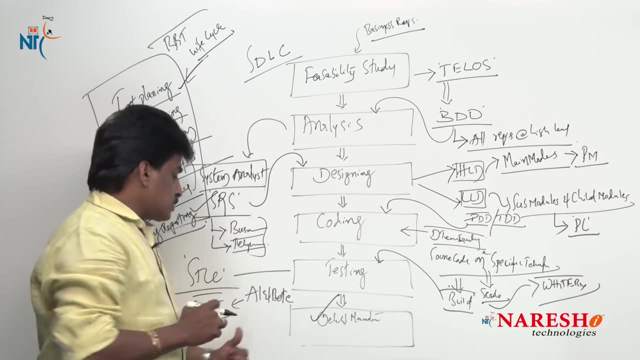 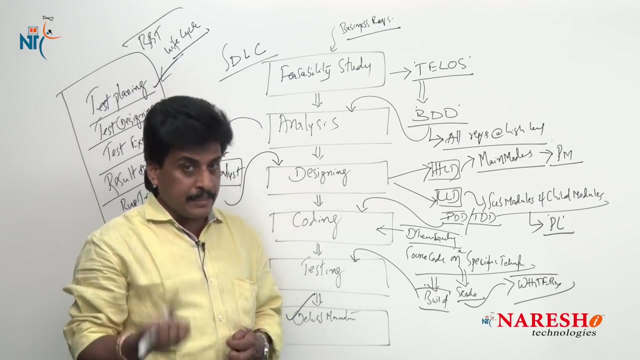 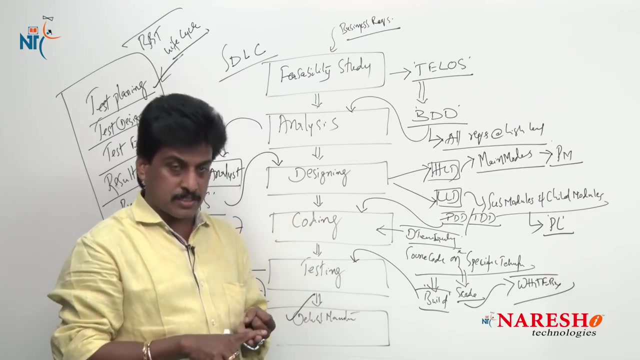 verifying their each and every application properly working or not within the company location. that is comes under alpha testing. once alpha testing successful, we are delivering the project to client, client checking now this application at the client environment area, so properly working or not, they are checking with their testers or third-party testers, the beta. 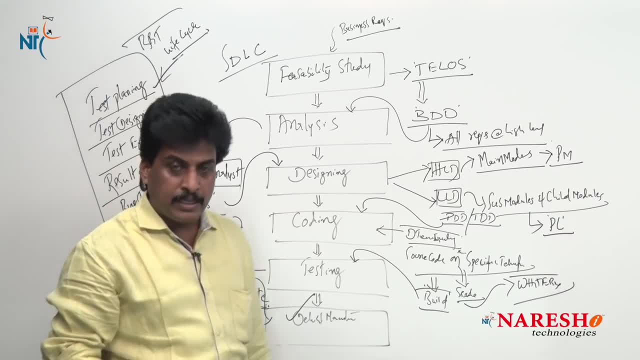 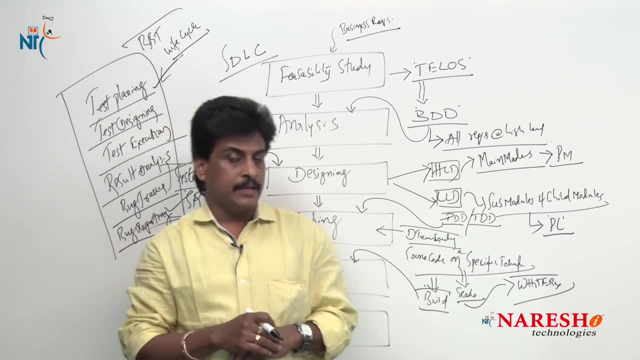 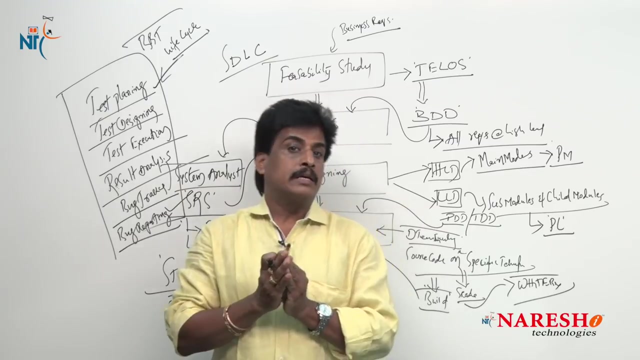 testing. once beta testing successfully completed, the delivery process will be closed. after that, maintenance will be entered. this maintenance again, free maintenance available, paid maintenance available or 50, 50 percent. we need to, according to the client environment, that is, the project, according to our client requirements level. whenever we bdd before, whatever the documentation, 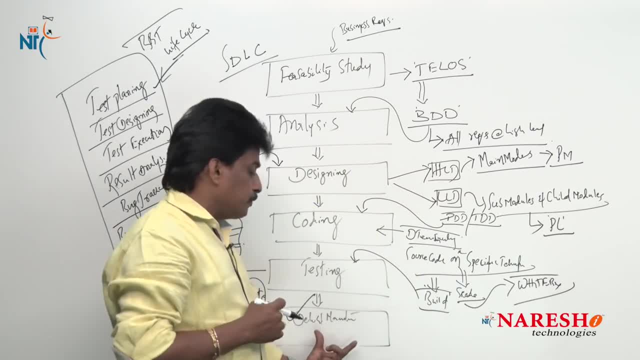 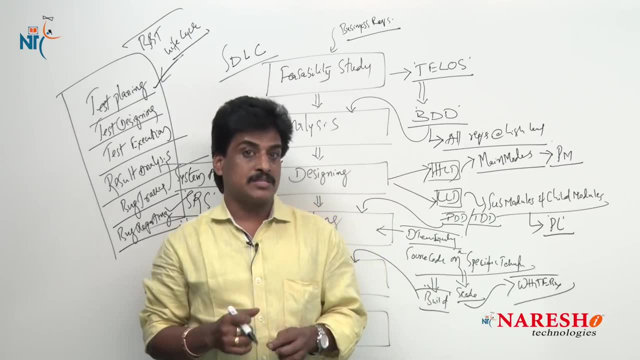 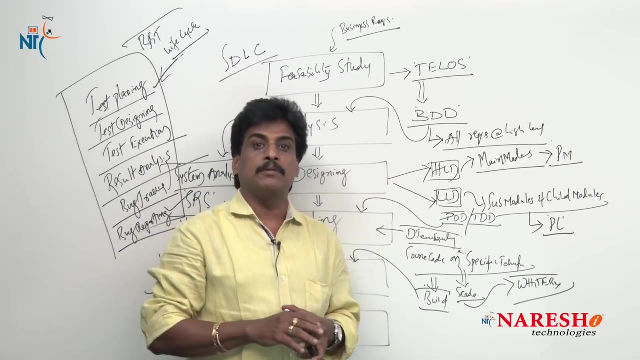 rules and regulation standards available. according to that, some rules will be entered in the maintenance. so according to that company giving maintenance to client. so this is total system development life cycle. you are related to any technology guy. you must know what is a system development life cycle. so each and every phase area. what are the exact components? 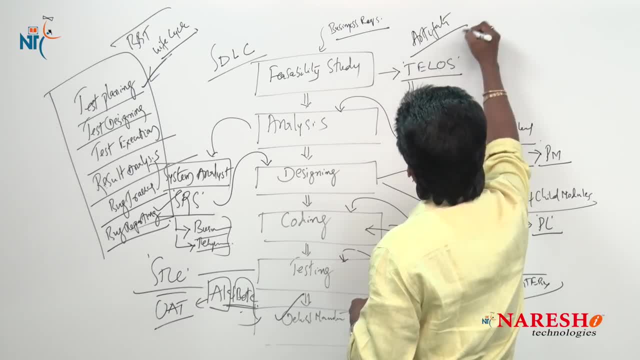 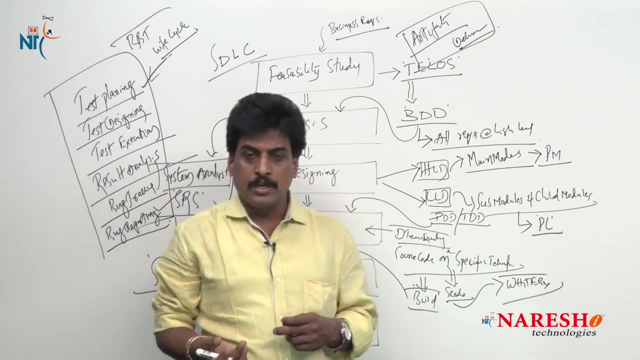 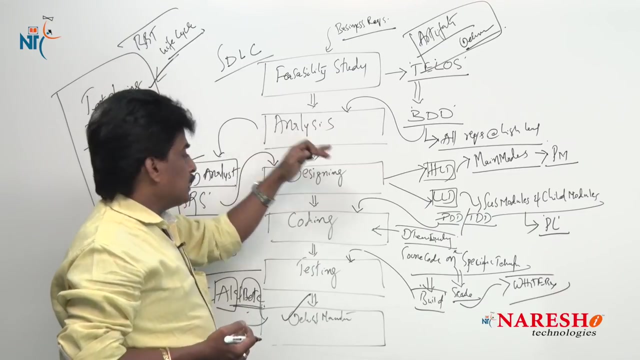 available, what are the components available, what are the components available, what are the artifacts available, what are the deliverables available. so each and everything explained very clearly: artifact is nothing but inputs, deliverables are nothing but outputs. so each and every person, business analyst team, system analyst team, designing means technical design, document is